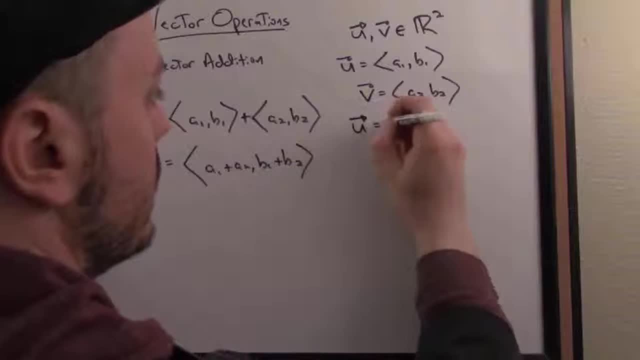 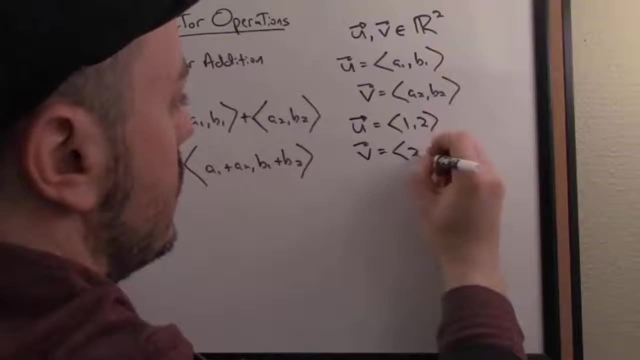 Let's just see a quick example with some numbers, just to make that nice and clear. So if we have the vector u, let's call it 1, 2, and the vector v, let's call it 2, 0.. 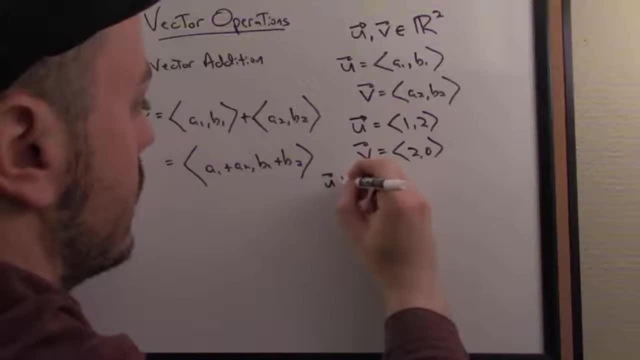 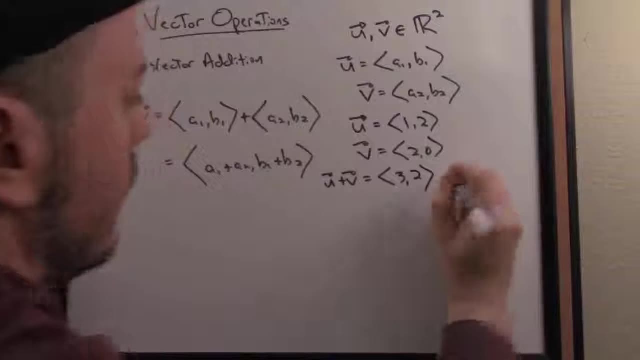 If I then wanted to add these two vectors together, I add them component-wise. So I got: 1 plus 2 is 3,, 2 plus 0 is 2.. There is my resultant vector, u plus v. Okay, So to make the resultant vector, I'm going to call it u plus v. 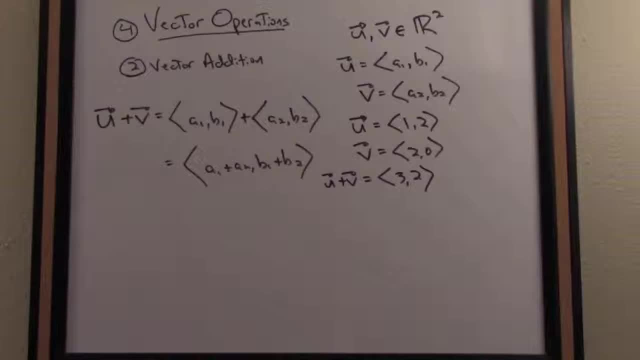 And I'm going to make this idea of vector addition in algebraic sense connect well with a geometric interpretation. Let's draw a geometric picture of vector addition as well. I have my vector u. Okay, let's draw it like this. Let's say there's the vector u- 1, 2 approximately- and the vector v. notice, it's just a horizontal. 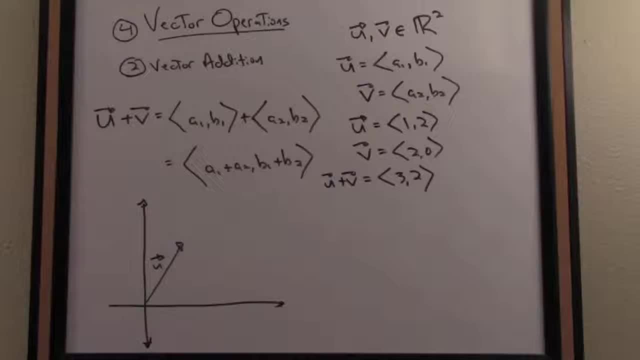 vector. Well notice, I can place v anywhere I want in the plane we defined. vector addition in a geometric sense is you align the vectors head-to-tail, head-to-tail in order. So I'm going to align these with u first and then v and the resultant vector when I add. 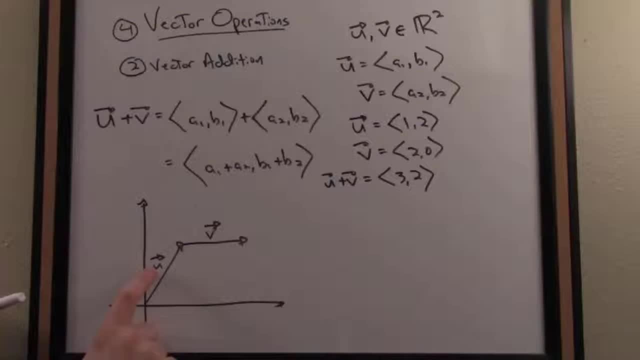 these together has initial point that aligns with the initial point of the first vector u and terminal point that aligns with the terminal point of the second vector v. So in other words, that vector in blue is my resultant vector. geometrically, u plus v Addition has a really 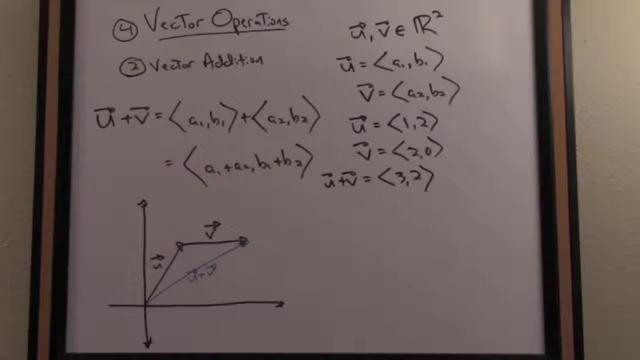 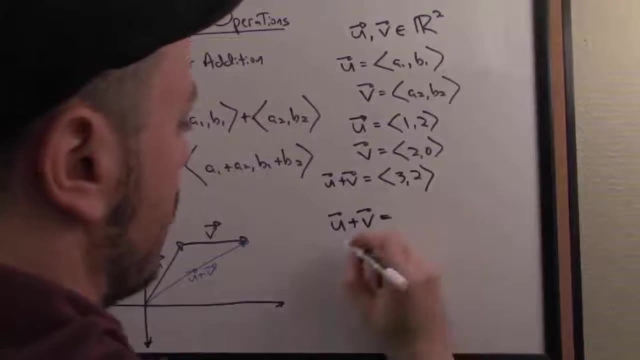 nice property that the order doesn't matter. So 1 plus 2 is the same as 2 plus 1,, for instance. right Well, that property extends for vectors. So in other words, u plus v is equal to v plus u. 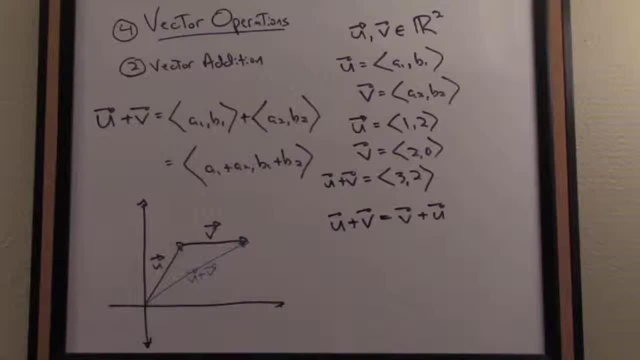 in the opposite order. This property is known as the commutative property of vector addition, In other words, the order in which I add the vector addition to the vector addition is the commutative property of vector addition, In other words, the order in which I add the vector addition to the. 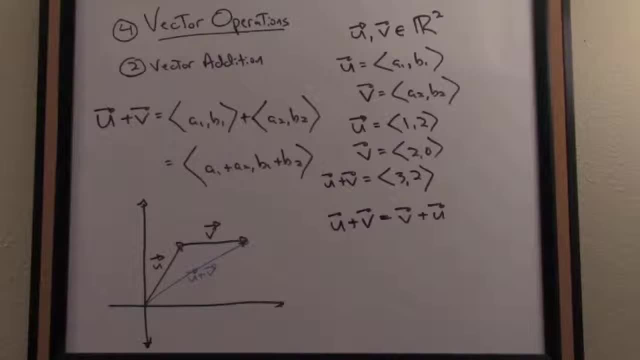 vectors does not matter. And why is that true? Well, in a basic sense, this property is inherited from the fact that when I add real numbers together, the order doesn't matter. So that's a nice property that we should also see reflected geometrically. So how would I then write v plus u? 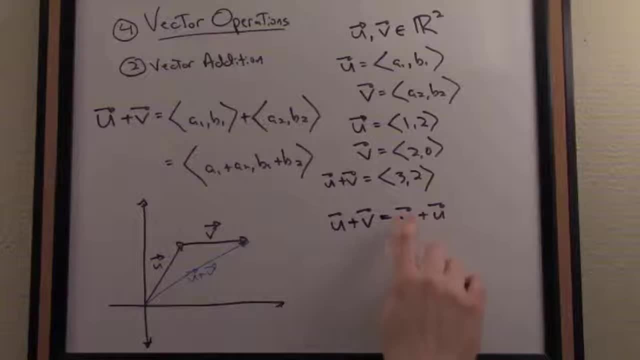 Well, I arrange the vectors geometrically head-to-tail. head-to-tail now, starting with v. So if you remember v, I can draw the equivalent vector 2, 0 anywhere in the plane, as long as it has the same direction and magnitude. So let's see that, Let's. 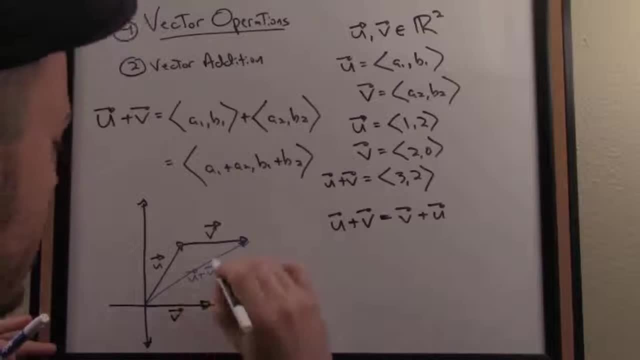 draw v here. So let's say there's my vector v and then I'm going to add to that the vector u here, which I've also translated, So as we can see v plus u, by definition, geometrically it has initial point at the beginning, vector v, and terminal point at 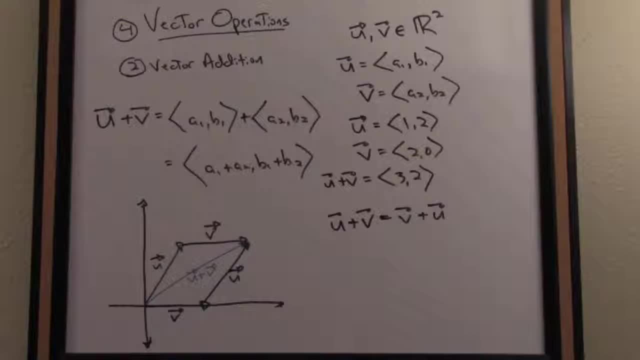 the end vector, which is now u, And of course, yes, we get the same resultant vector. Now, this nice picture is sometimes called the parallelogram law of vector addition. In other words, if I draw a parallelogram, I'm going to get the same resultant vector And I'm going to get the 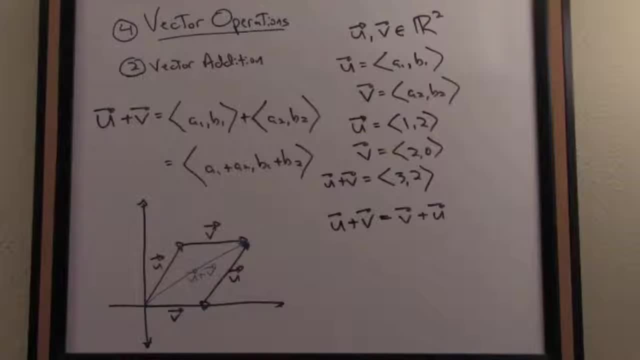 parallelogram using vectors u and v as the outer edges. The long diagonal of that parallelogram represents the sum of the two vectors, u plus v. 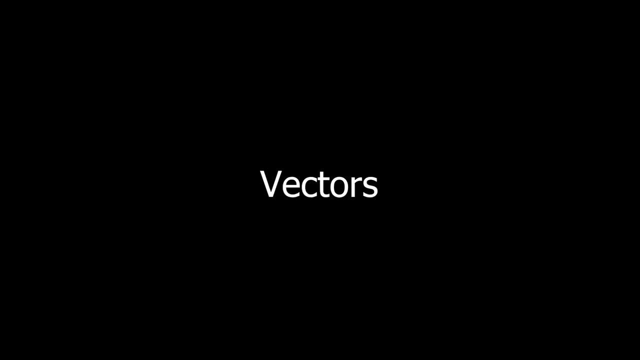 This question says: write the vector a to c in terms of a and b. So a to c means from a to c, So we need to go from here up to here. Now we can't actually go along this route because it hasn't got a name. We don't know what it's called, So we need to go a different. 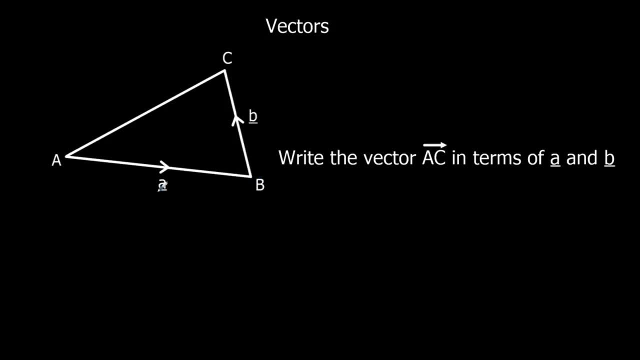 route We can see that a to b is called a. So the route a to b here is called a And the route b to c that's called b. If I went backwards along a to b, if I went from b to, 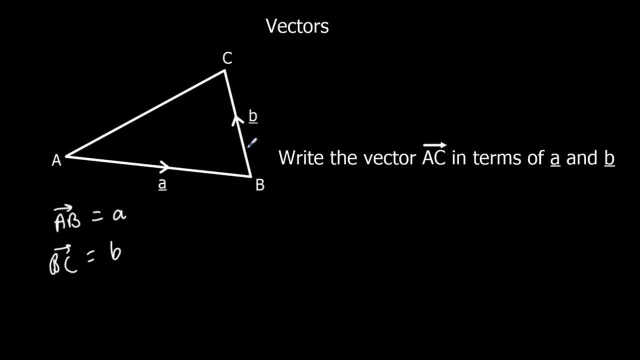 a, that would be a minus a. If I went from c to b, that would be a minus b. But to go to a to c, I'm going to go from a to b. So I'm going to go a to b, which is an a.